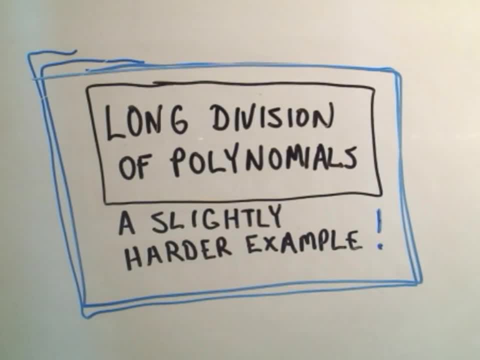 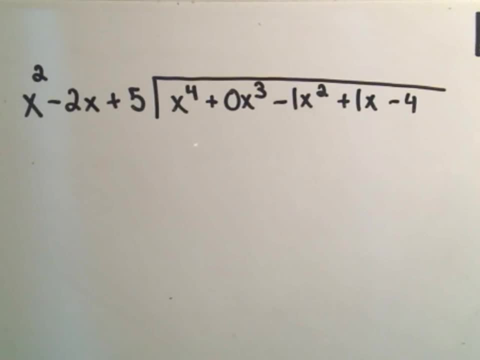 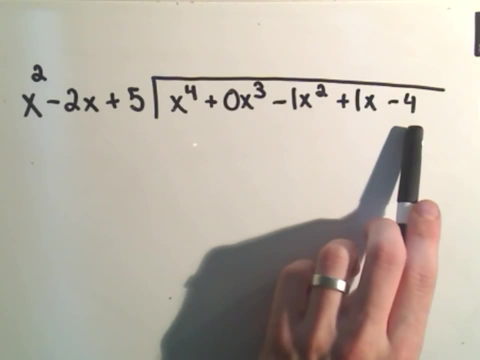 Okay, in this video I want to do another long division of polynomials. An example that's maybe a touch harder than the other ones. I had a couple requests, So this time we're going to take the polynomial x to the fourth plus zero, x cubed, minus x squared, plus x minus four- I think my country accent came out there for a second. We're going to divide all that by x squared minus two, x plus five. Okay, so again notice, underneath there is a 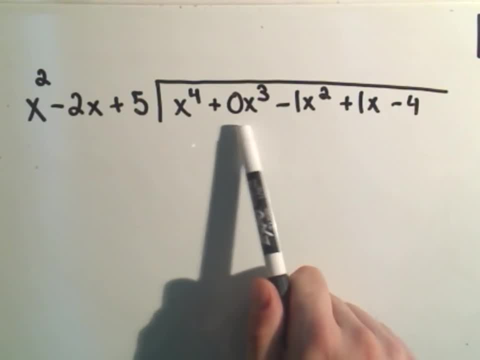 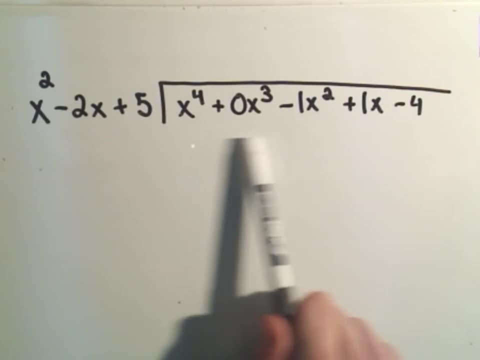 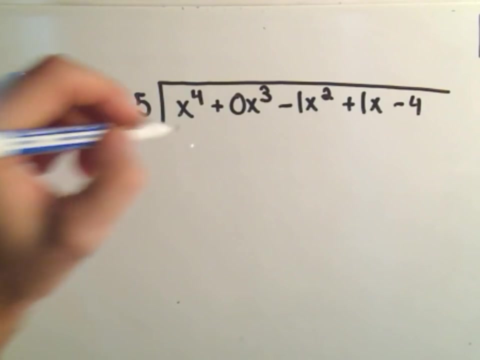 Even though there wasn't an x cubed term, I went ahead and filled in the zero x cubed just as a placeholder. You know all this is going to do again is just help you keep, I think, things lined up. Notice also it's in descending order. So fourth power, third power, second power, first power in our constant Same thing on what we're dividing by on the outside. Again, you just focus in on the highest powered things: X squared and x to the fourth. 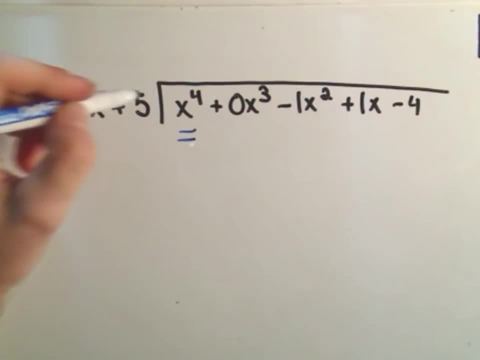 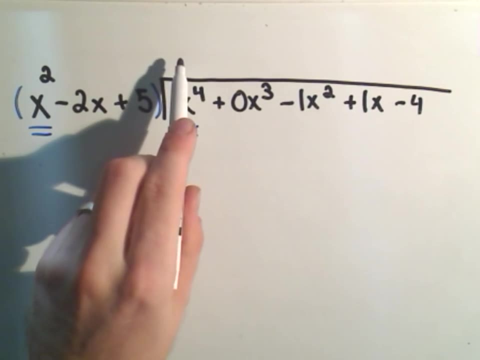 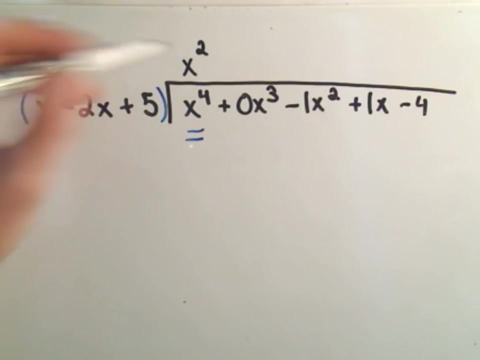 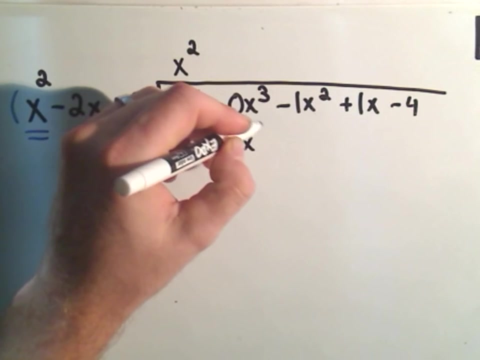 And usually something I always did too, is I went ahead and put my stuff in parentheses just to remind myself to distribute everything out. Okay, so I think x squared times what is x to the fourth? Well, I'll need another x squared when I do that. So I have to distribute everything x squared to everything. So I'll get an x to the fourth term. I'll get minus two x to the third. Looks like I'll get positive five x squared. 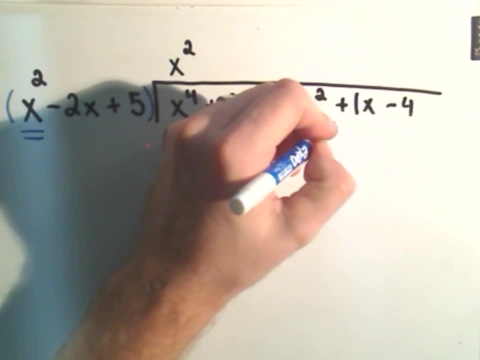 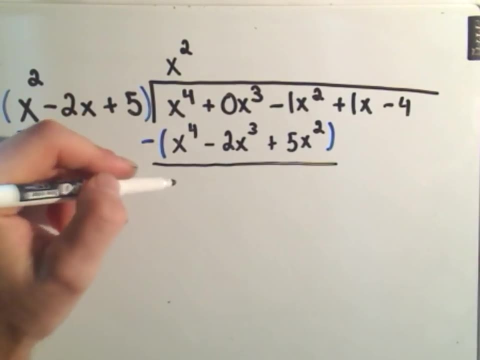 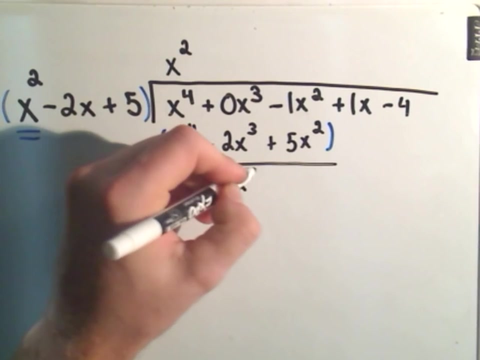 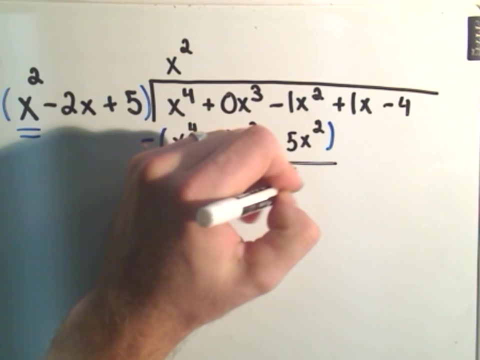 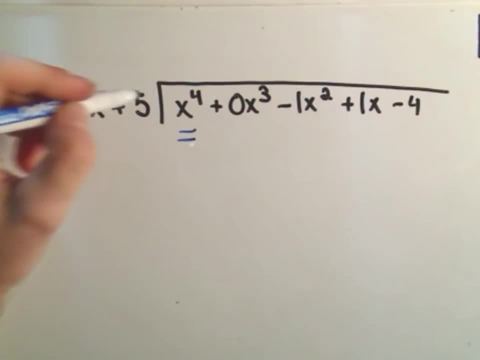 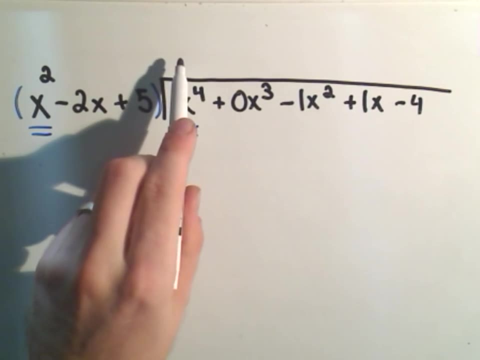 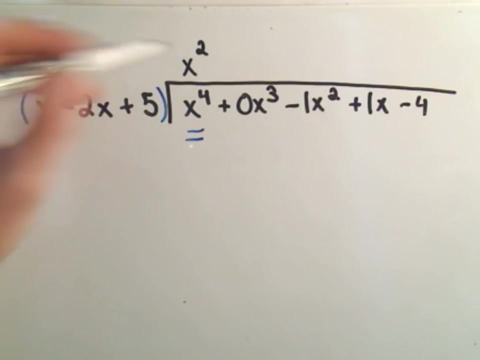 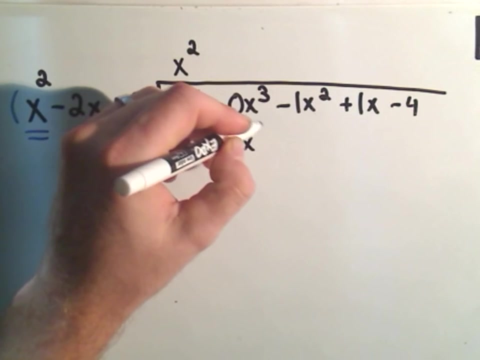 And usually something I always did too, is I went ahead and put my stuff in parentheses just to remind myself to distribute everything out. Okay, so I think x squared times what is x to the fourth? Well, I'll need another x squared when I do that. So I have to distribute everything x squared to everything. So I'll get an x to the fourth term. I'll get minus two x to the third. Looks like I'll get positive five x squared. 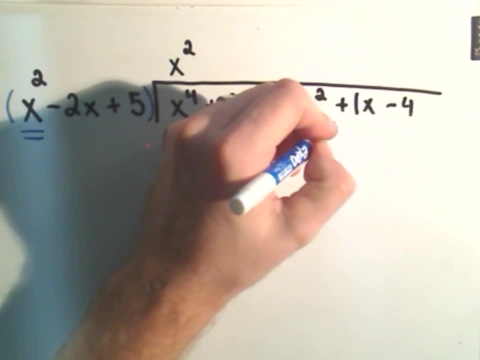 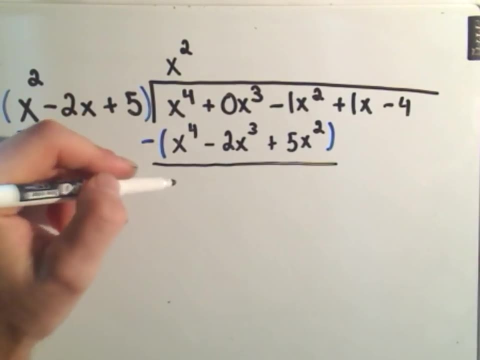 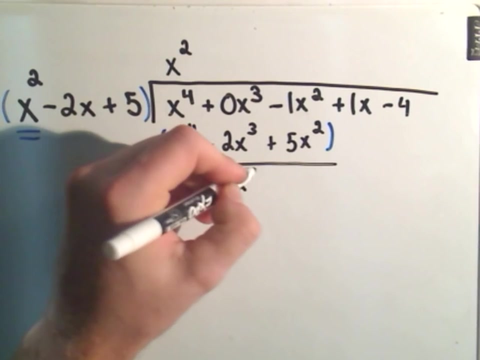 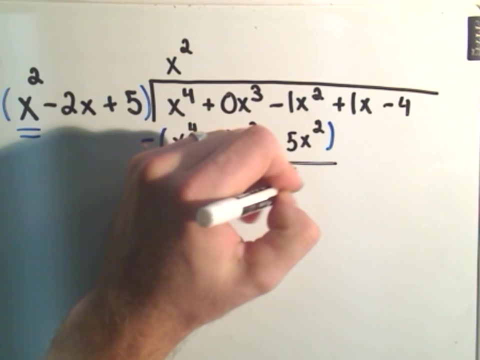 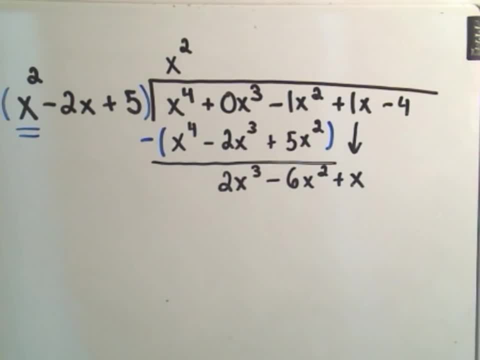 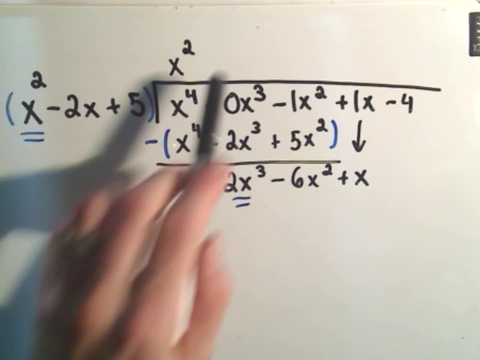 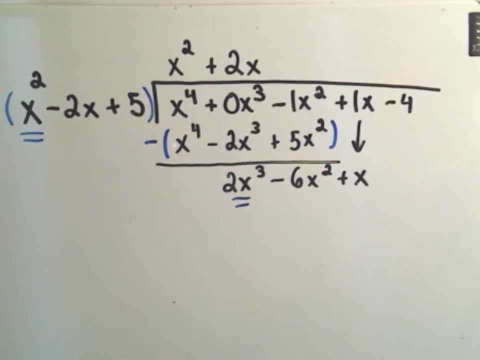 x. and then now I play the same game. I look at my x squared and I look at my highest power term and I think, well, x squared times, what is going to give me 2x to the third? Well, I'll need a positive 2 to get the 2, and then I believe I'll need an extra x to 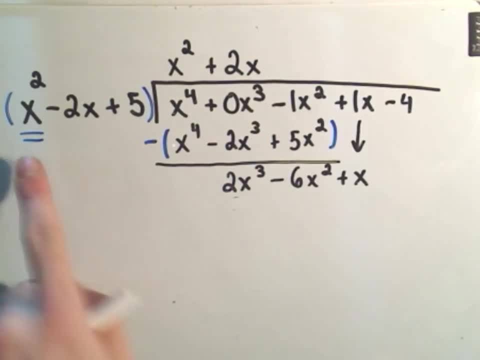 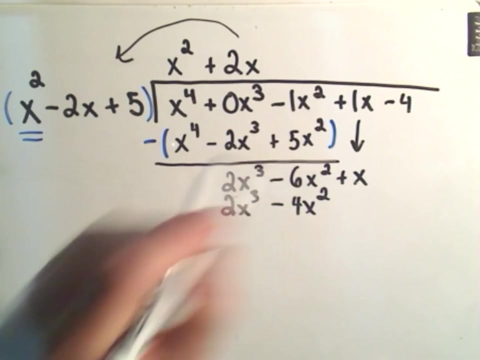 get that x to the third power. Okay, so again, 2x times x squared is going to give me 2x to the third. So again now I distribute this guy by everything in the parentheses, so I'll get 2x to the third. It looks like we'll get negative 4x squared and then we'll 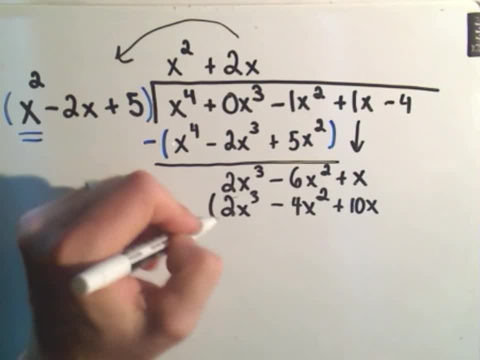 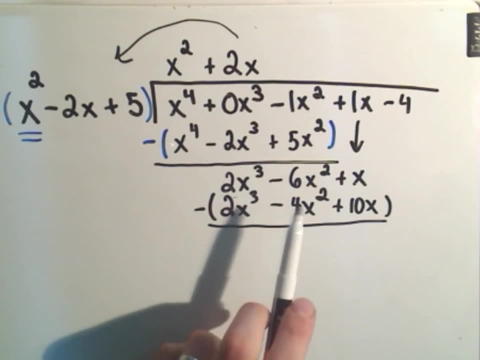 get a positive 10x. Again, I do the same thing. I just put it in parentheses and subtract it out. so the 2x cubed will cancel out. I'll get negative 6x squared plus 4x squared. so 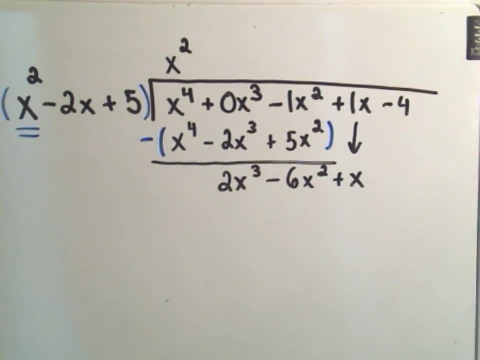 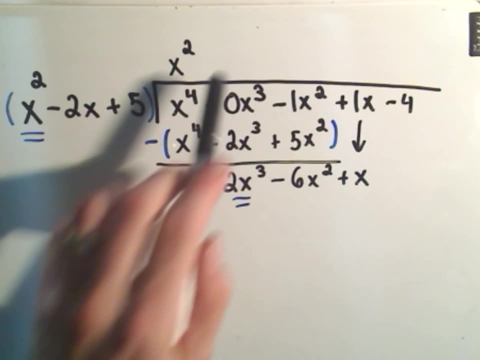 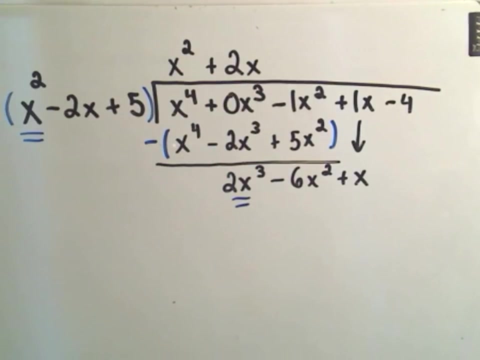 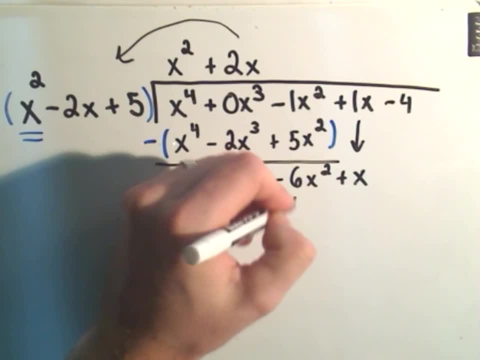 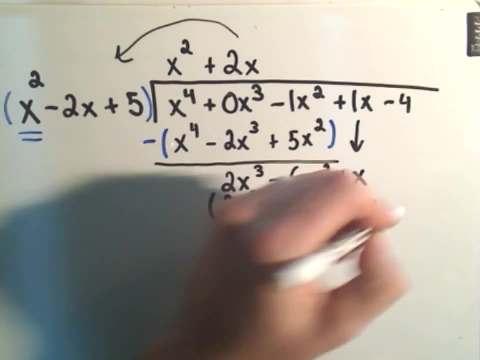 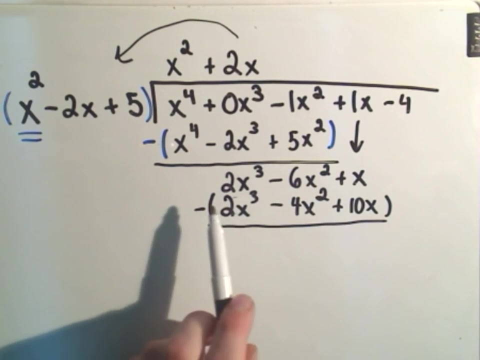 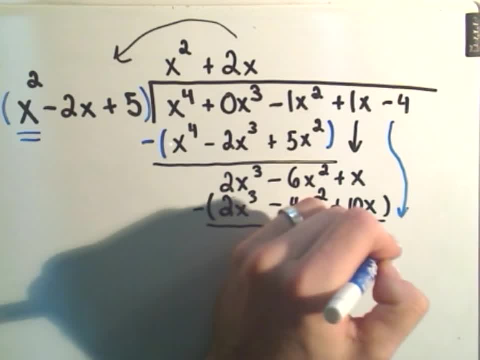 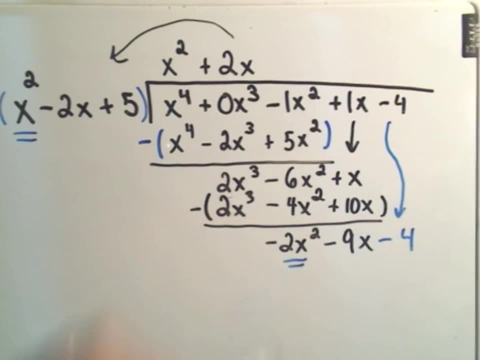 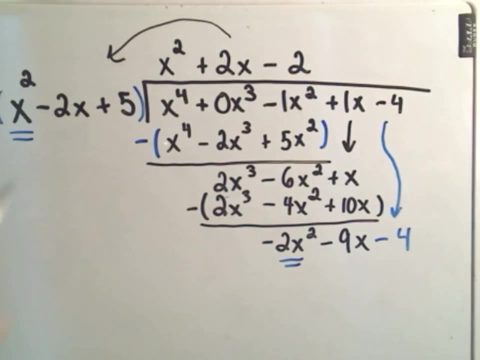 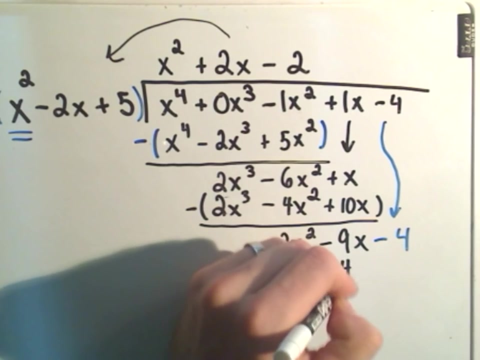 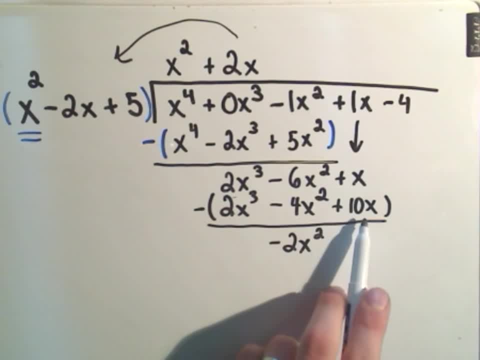 that's negative 2x squared. I'll have x minus 10x, so that's negative 9x. and then I'll get negative 4x squared, so that's negative 9x squared. I'll have x minus 10x, so that's. 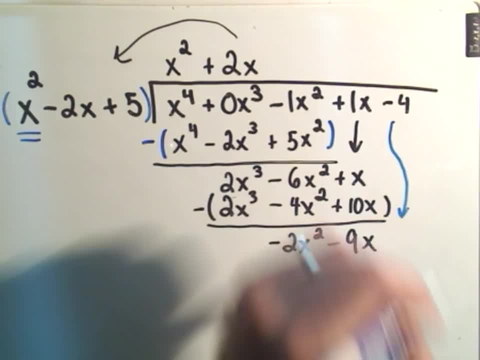 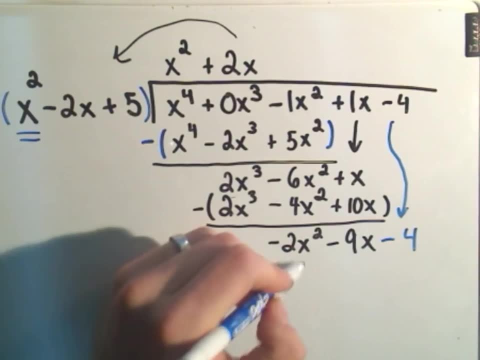 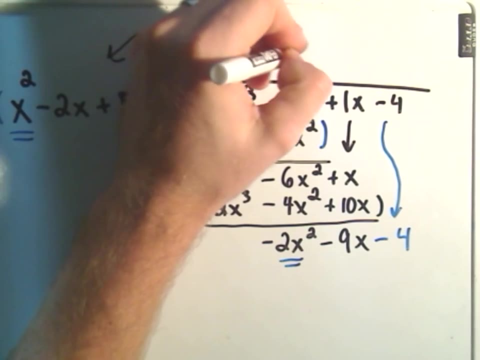 negative 9x squared. And again I drop my number down, my minus 4.. Okay, so that'll be the new part. Again, now I look at the x squared and the negative 2x squared and I think, well, x squared times, what is negative 2x squared? I'll need a negative 2.. So again, 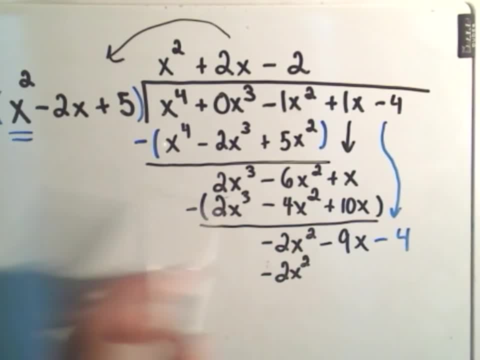 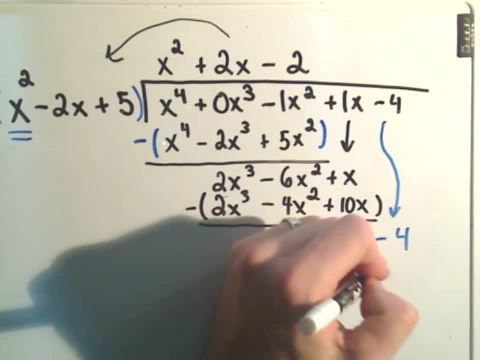 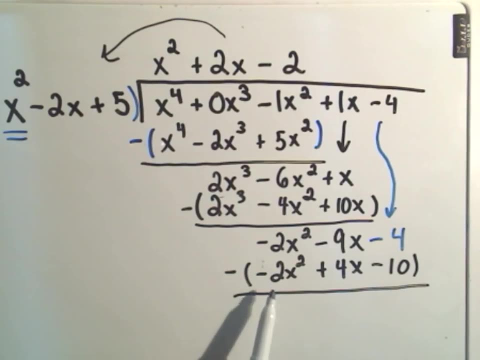 when I multiply, I'll get negative 2x squared. I'll get positive 4x. I'll get negative 2 times positive 5, which is negative 10. Again, I put it in parentheses: subtract: I'll get negative 2x squared plus. 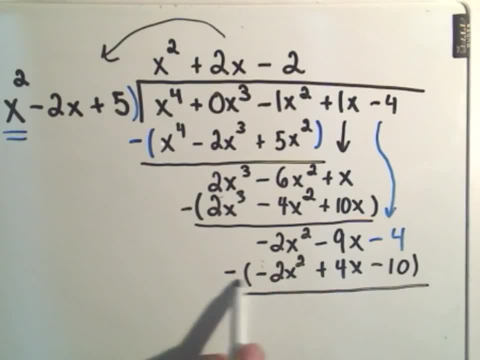 2x squared, which is 0x squared, I'll get negative 9x minus 4x. That'll give me negative 13x, And then I'll get negative 4 plus 10.. Negative 4 plus 10 is positive 6. And once. 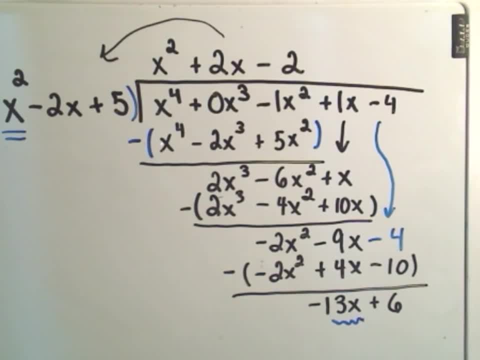 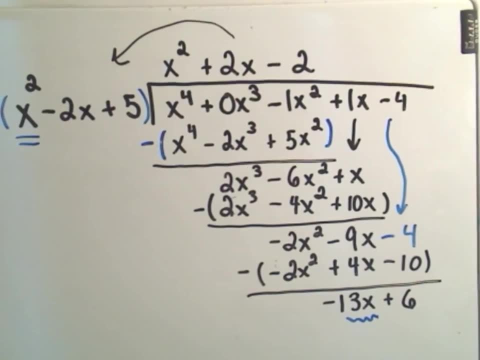 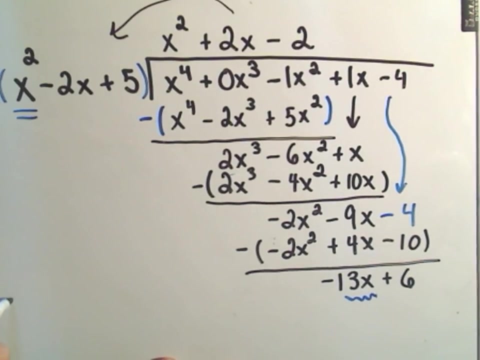 you look at the highest power of the thing that's remaining. once the degree of that is smaller than the degree of the highest power thing that you're dividing by, you are finished. Okay, So we've done all the long divisions. So really it says: what we have here as a result is we can write polynomial. So we were starting with- I didn't write it out- but we had x to the 4th minus x squared, plus x minus 4.. That's the thing I put underneath. We're dividing by x squared minus 2x squared. 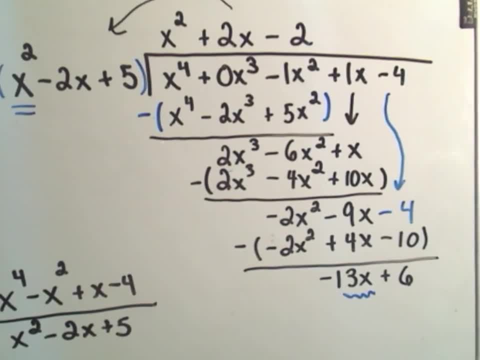 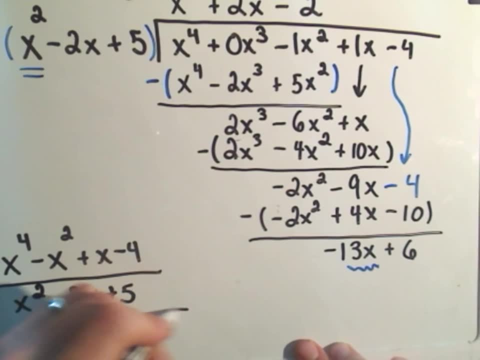 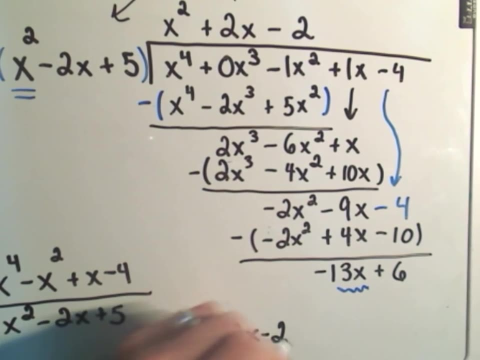 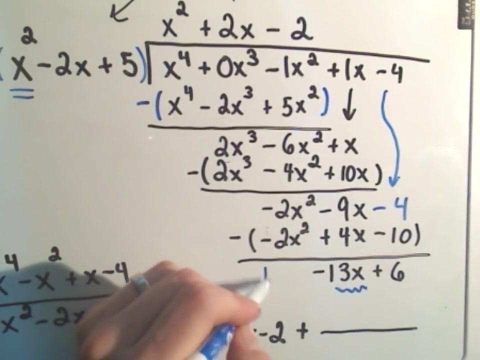 Plus 5.. And it says what all of this is going to equal to at the end. It says all of this is going to equal what we got on top, which is x squared plus 2x minus 2 plus okay, this is going to be your remainder, just like with normal long division. So our remainder is negative 13x. 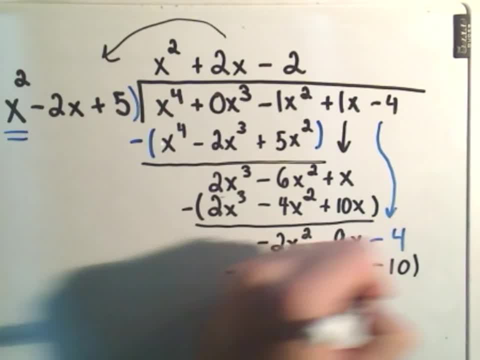 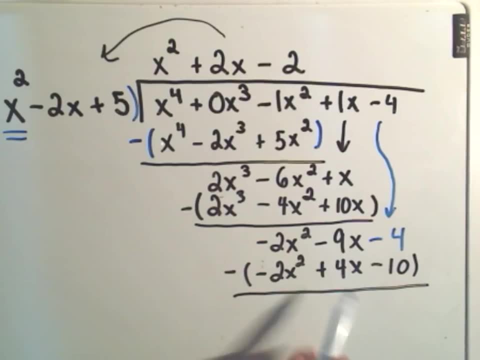 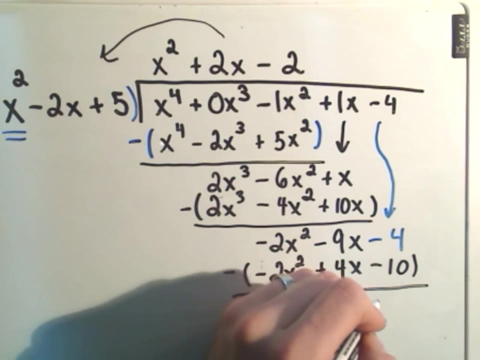 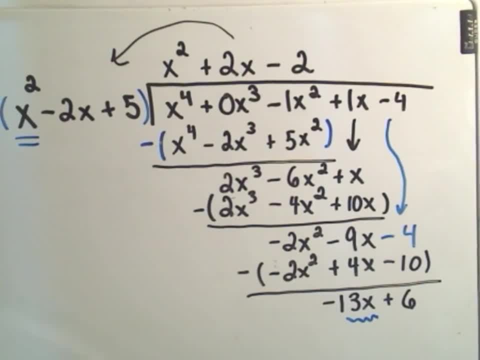 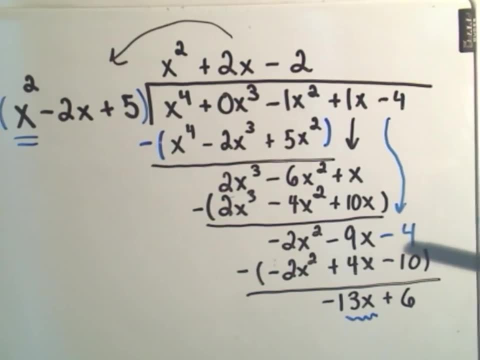 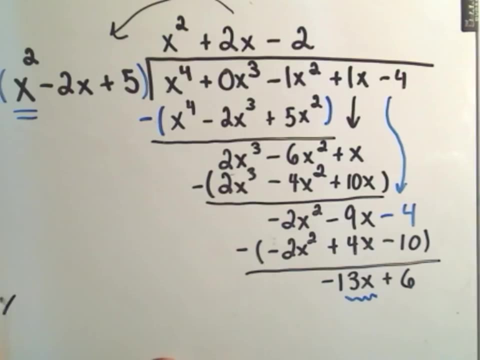 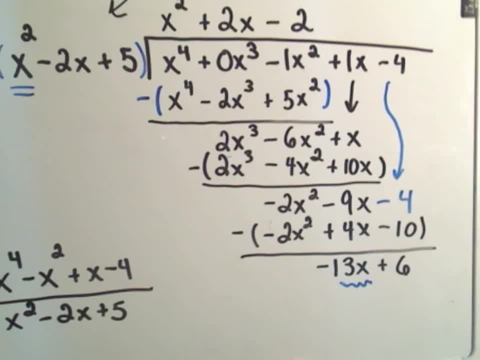 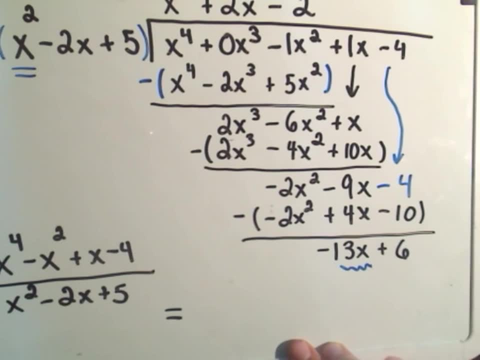 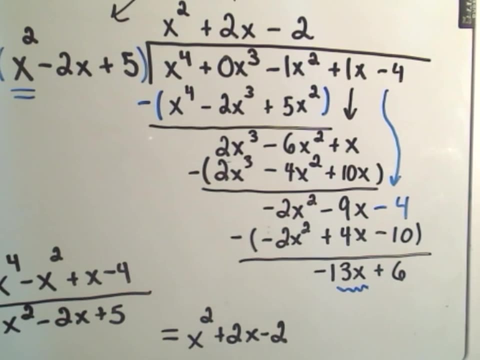 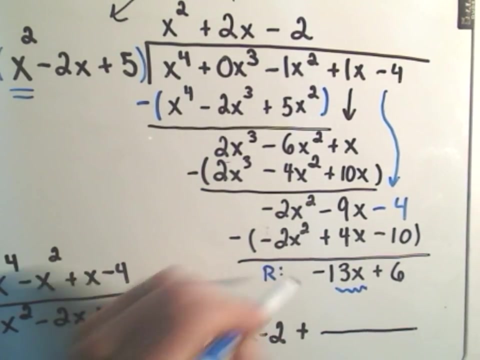